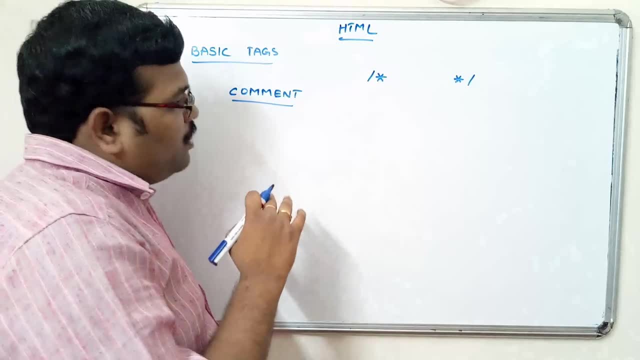 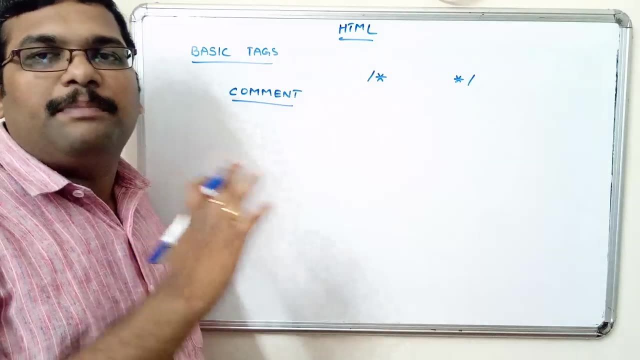 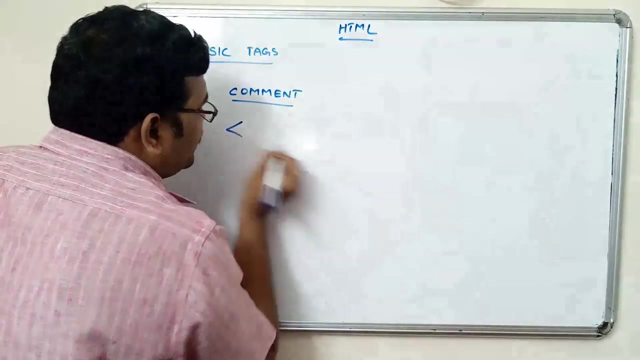 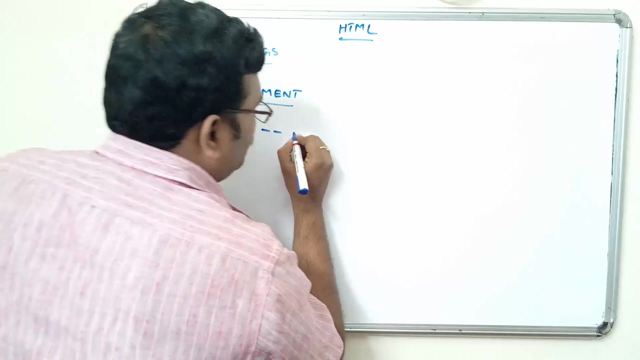 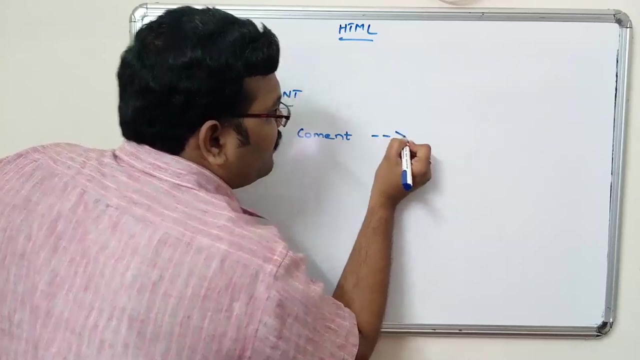 in between these two symbols. similarly, here also there are there is a comment tag right. so where the browser will not execute that particular statements. so in this comment, I mean in this HTML- the comment is represented as exclamatory mark: hyphen, hyphen. write the comment hyphen, hyphen and close the tag. so this: 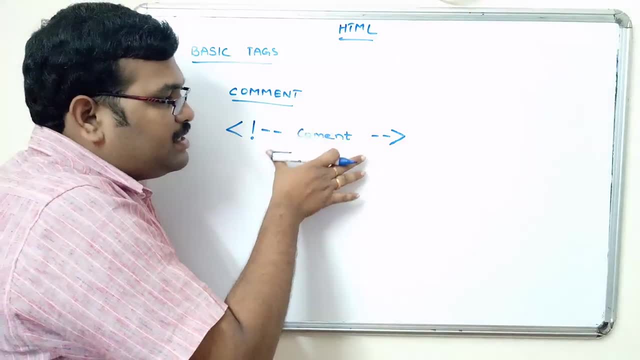 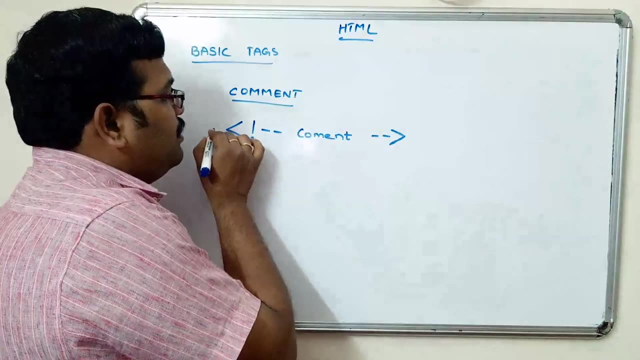 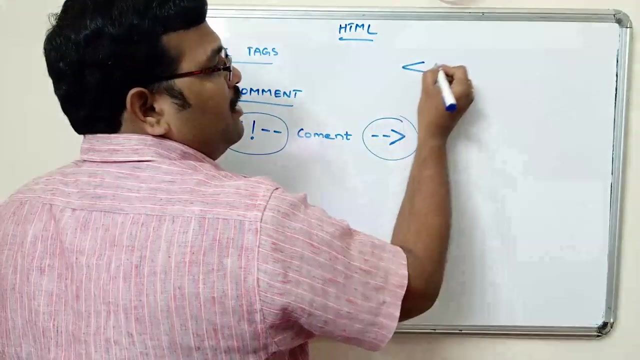 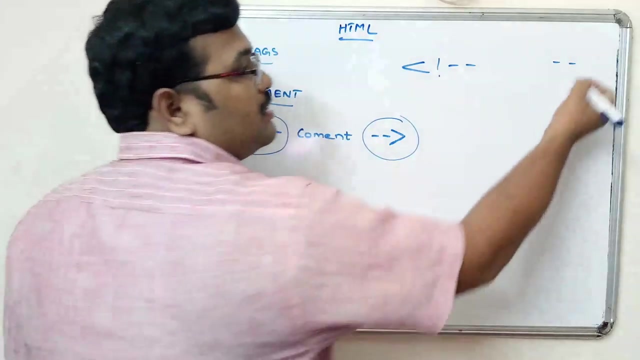 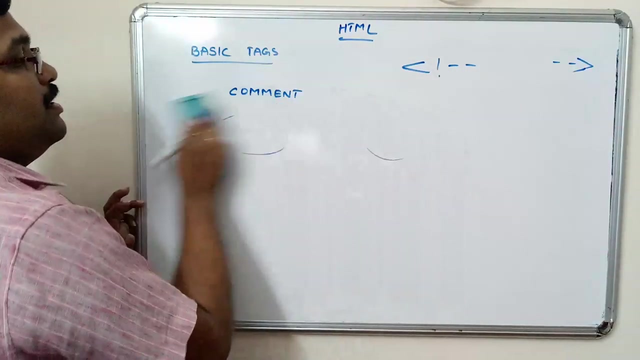 is the comment. I mean, this is the structure to write the comment in HTML. so, whatever the comment we are going to write, we should return in between these two symbols so less than exclamatory mark, hyphens. write the comment and hyphens close the tag. that means greater than symbol. right next, let 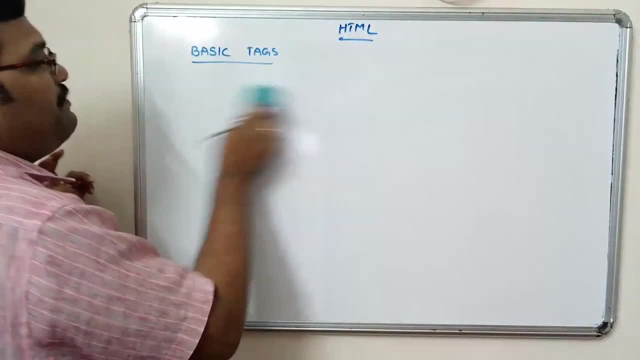 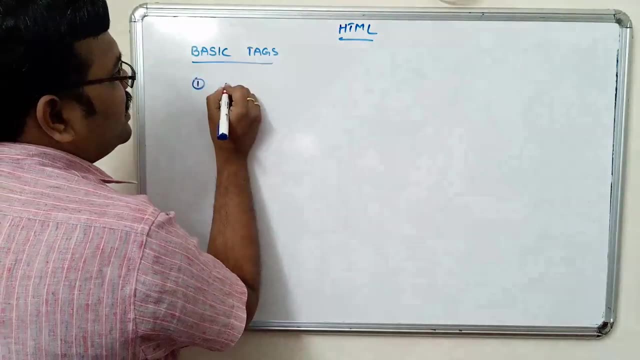 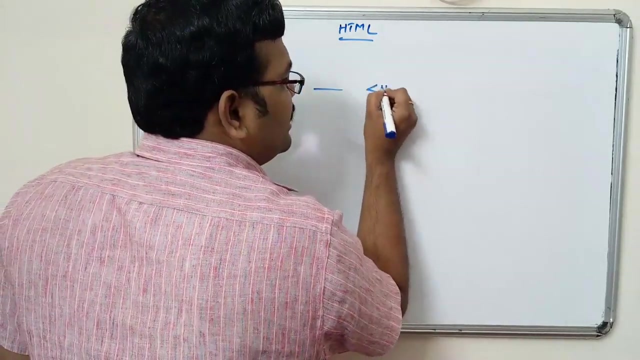 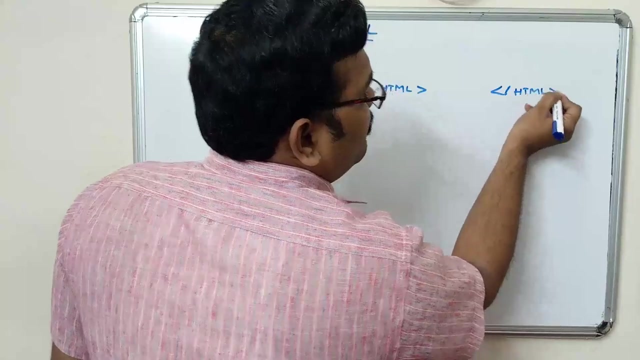 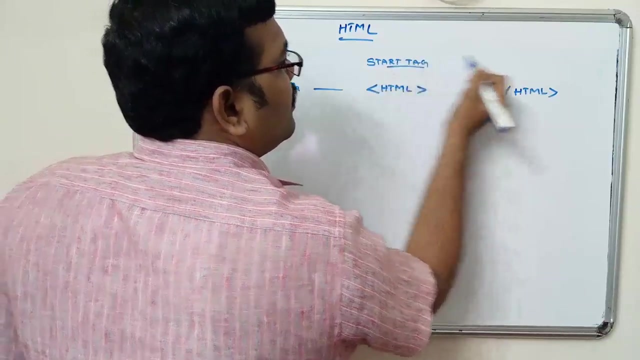 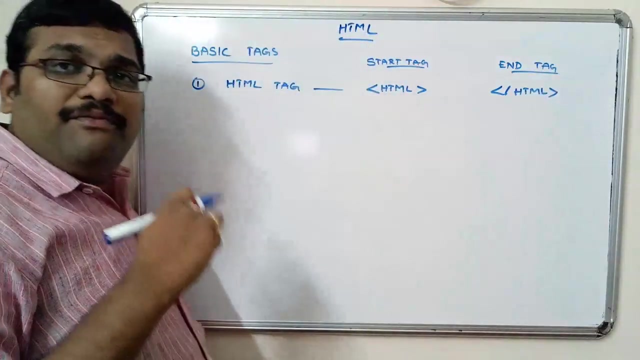 us see the basic tags. the first, very first thing is: every HTML page will start with the HTML tag. the first one is HTML base, so the starting tag is HTML. the end tag is slash html, right, so this is the start tag. this is the end today. so every web. page will be starting with HTML, so let us see the various tags about HTML and so each web page, the 육 when an HTML that we have немнож운데 tag, so it goes as long as it is a unetta √en tag tag, is one off, and this is so we have. número de let go. vamos de los corres. мы gun الق orbitando Nicholi. 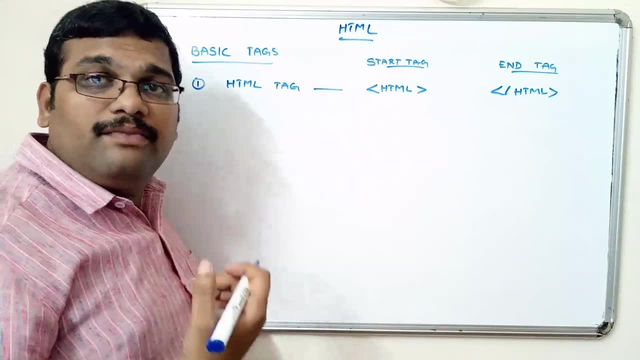 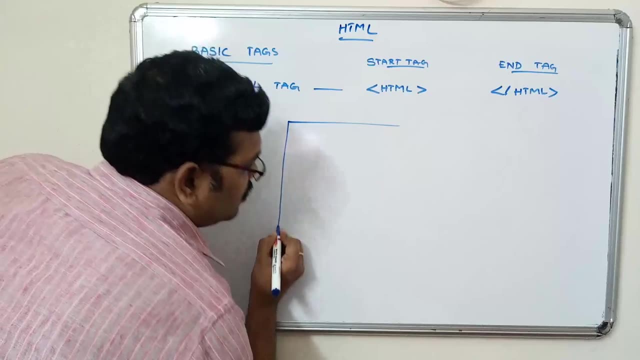 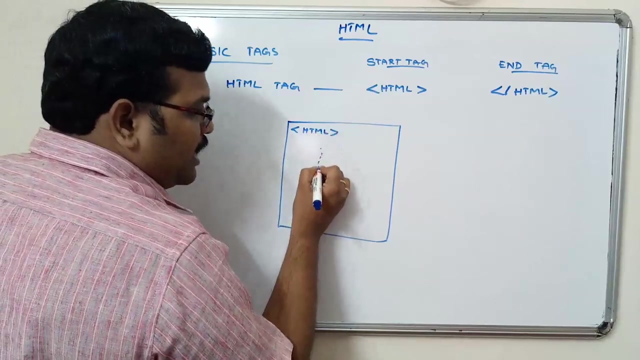 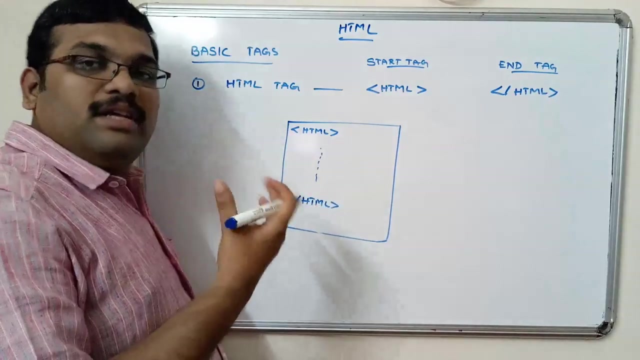 with HTML tag. so whatever the content we are going to write, that must be in between these two see. so, with the help of text editor, we will write the tags. so HTML write out the content after writing the content. close the HTML tag. so whatever the text we are going to write, that must be written in between these. 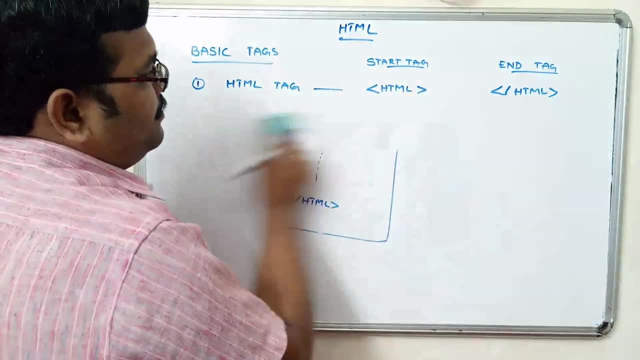 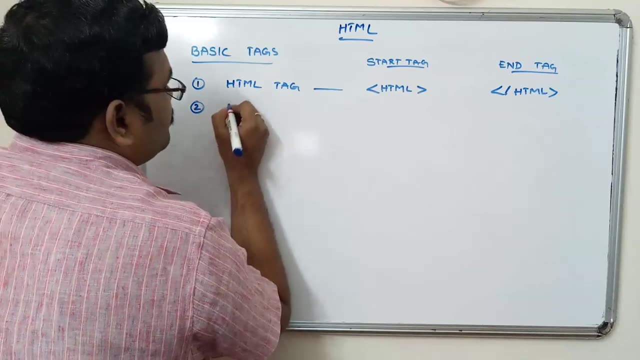 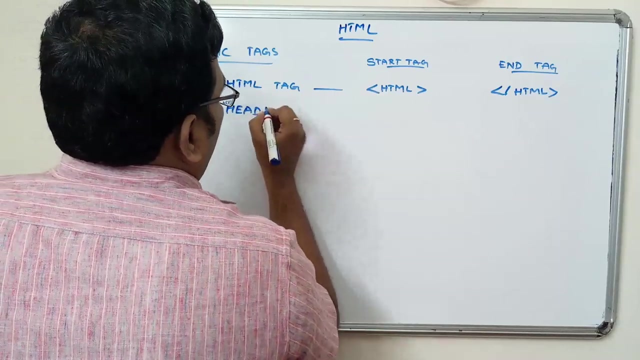 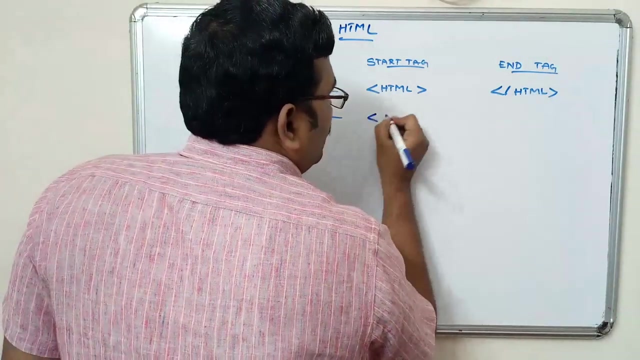 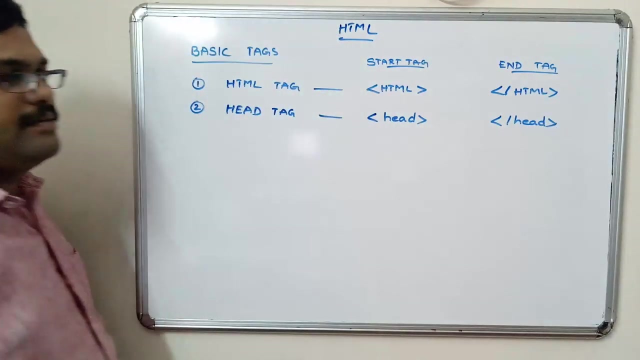 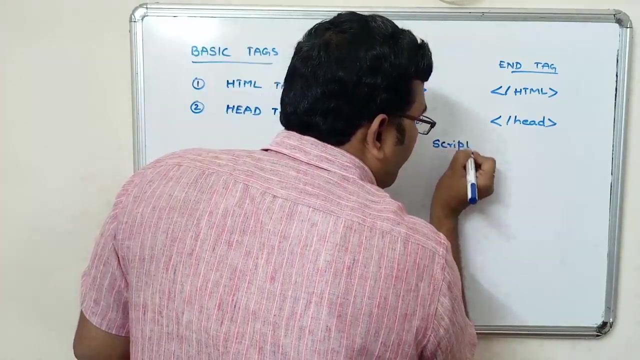 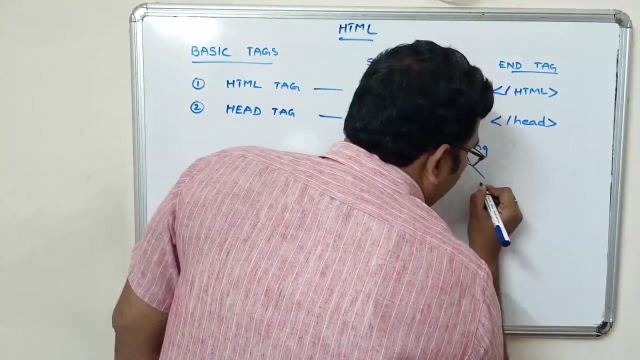 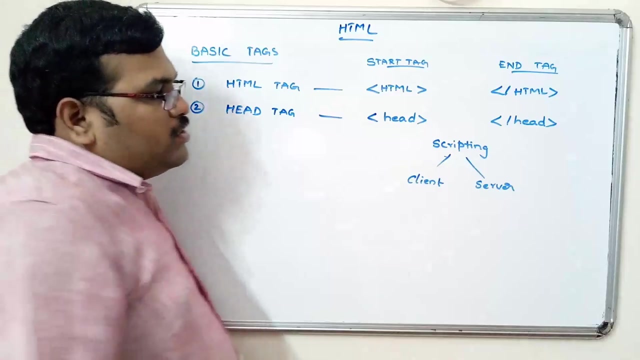 two text right next, the second, one head tag. here we have an HEAD, the starting tag, the ending tag and the end tag, backslash HEAD, and we will write the scripting, the client side scripting, both the client side scripting and the server side scripting. everything will be written in between this head tag, right? so what is the use of scripting? this is: 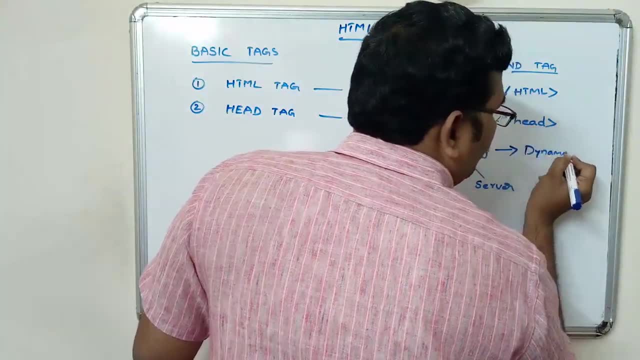 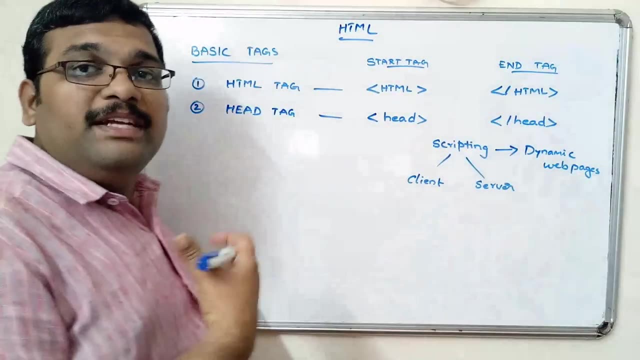 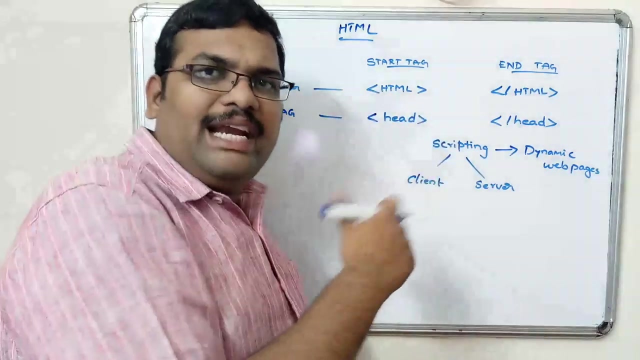 can be done for dynamic text webpages to create dynamic webpages. so time to times that data will be changed, right? so dynamic webpages. so we will see elaborately about these dynamic webpages and the static webpages in the next sessions, right? so just a note down that head. what is the purpose of head in? 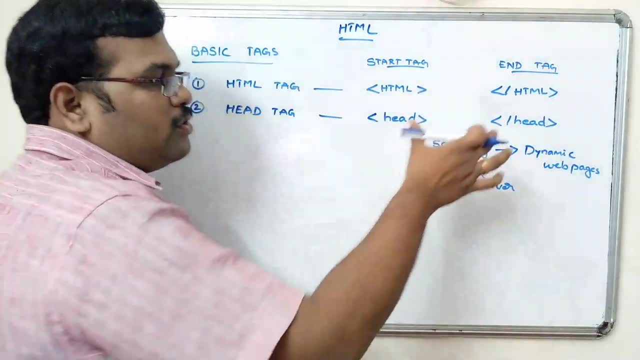 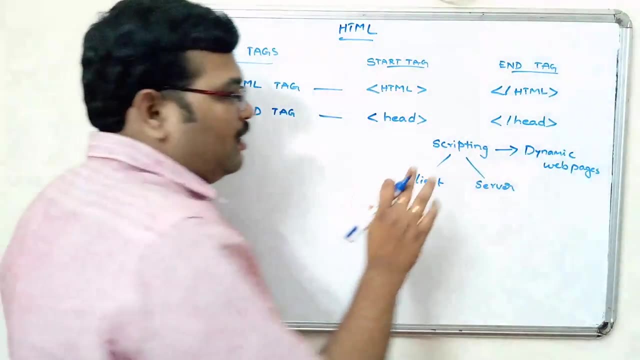 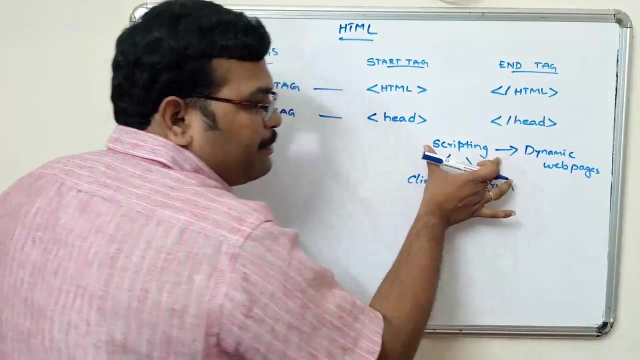 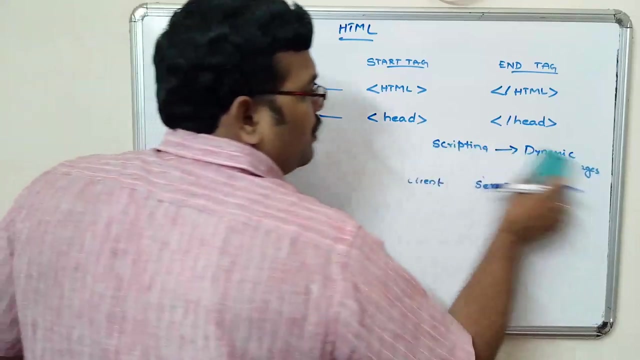 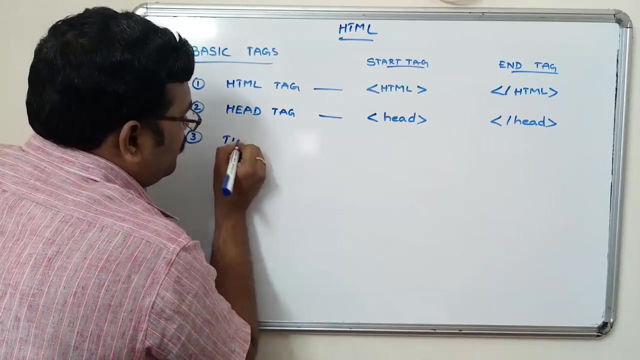 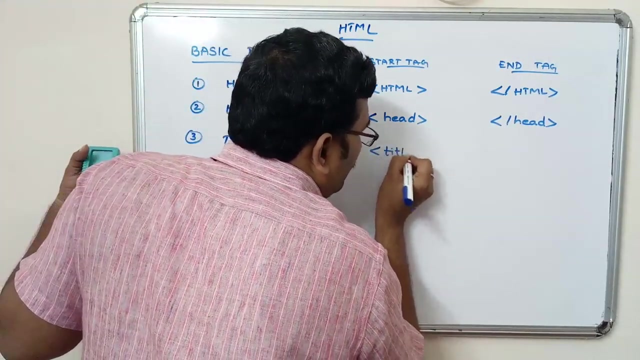 between his head tag. we will write the scripting. so scripting means client server, so both there are two types of scriptings: client side scripting and server side scripting. so both the scriptings will be written in between the head tag. so the main purpose of writing the scripting is to create the dynamic web pages. next title: is there for this? I think any tag. 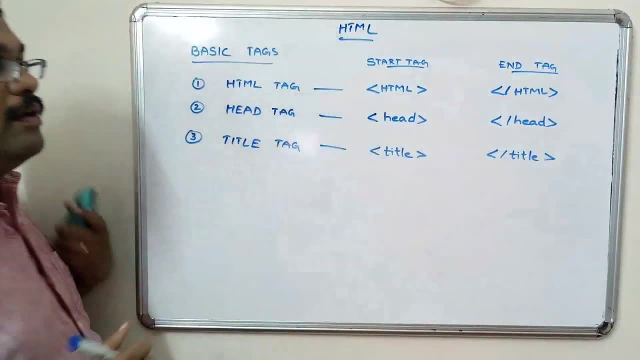 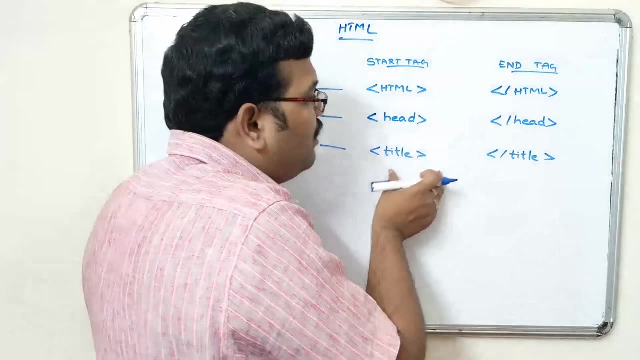 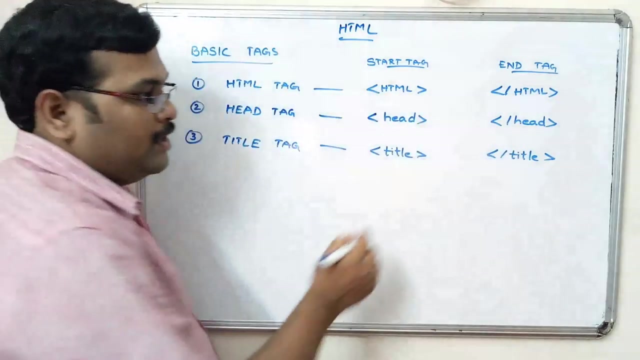 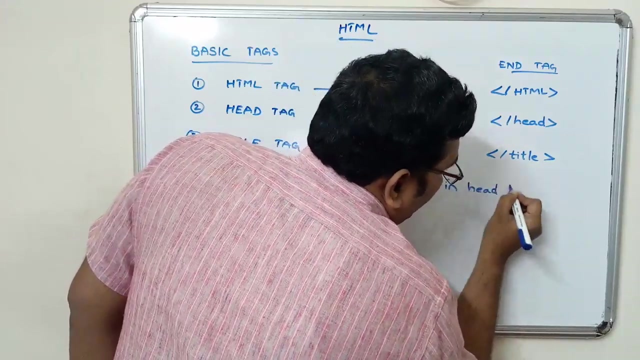 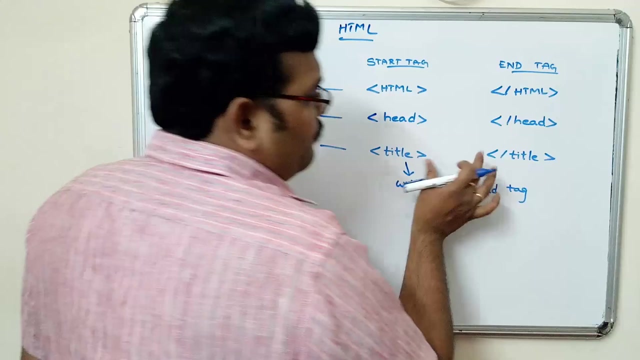 is slash title right. so well, well, we use this title tag, so this title tag is also a sub tag of head. that must be. I mean, this title tag should be written in between the head, so this must be written in head tag, right? so what is the purpose of writing this title? so, whatever the content we have, we are 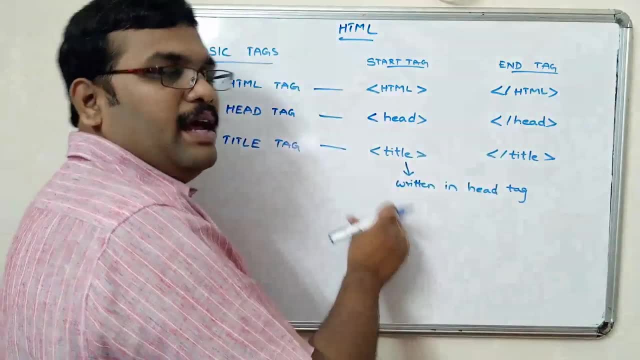 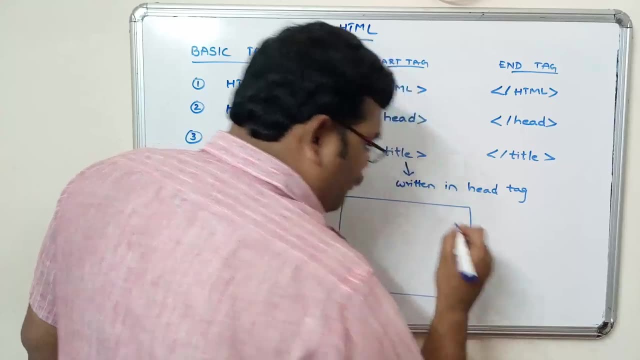 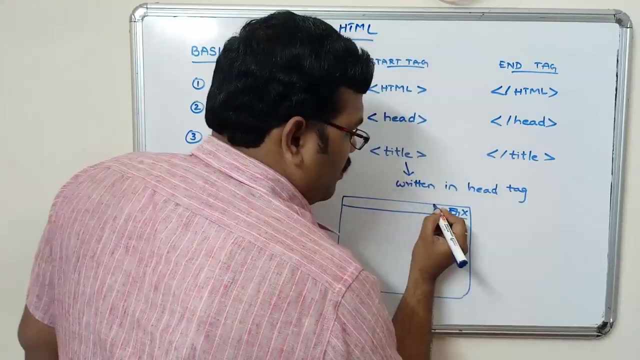 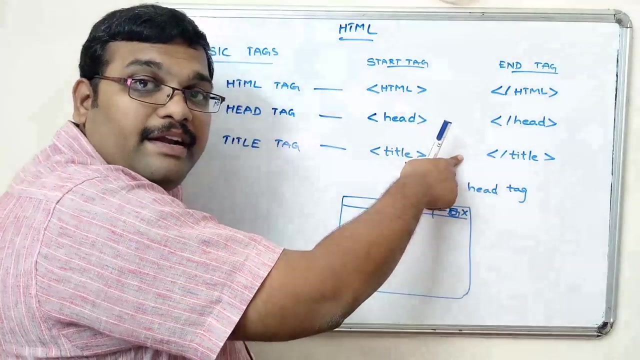 writing in between. this title, that will be printed as a title. that will be displayed as a title. see, let it bring. so if you open the web browser, so we can see this one, right. so web browser, so whatever the text we are writing here, that will be treated as a title. so here the title is this one. this is called the. 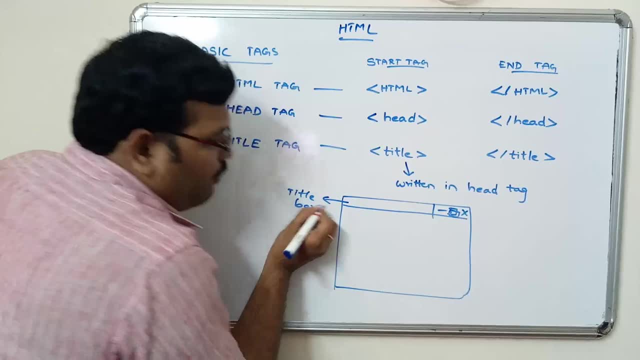 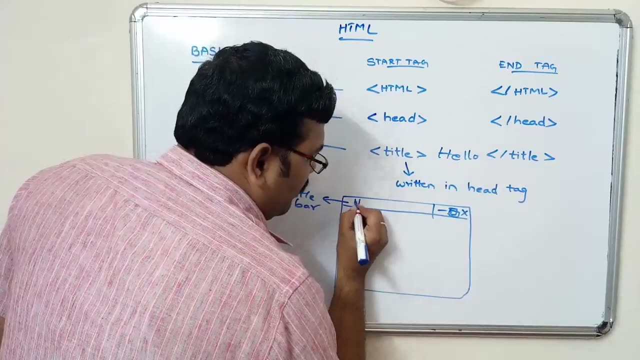 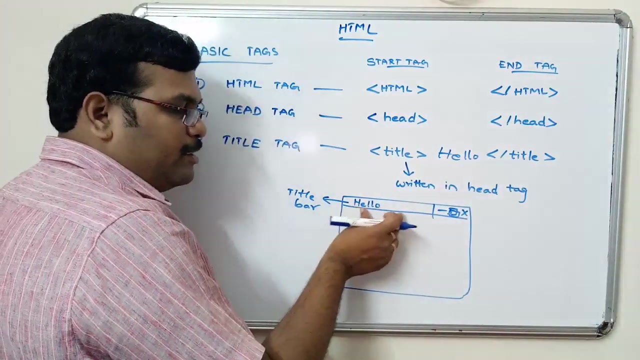 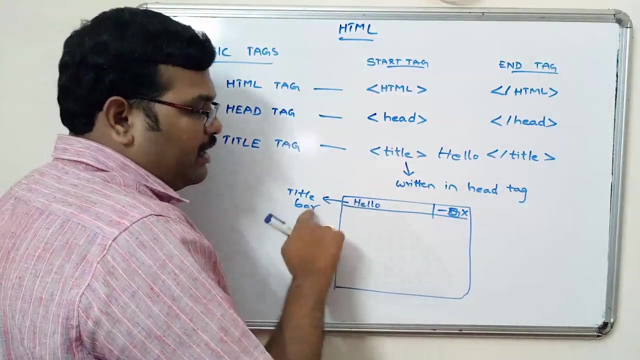 title bar. title bar. so whatever the content we are writing here, that will be printed here. so if you write hello, that will be printed in this place. hello, if you write here, welcome here, the welcome will be displayed in the title bar. so this is the web browser opening the. when you open this web browser, the tie in the 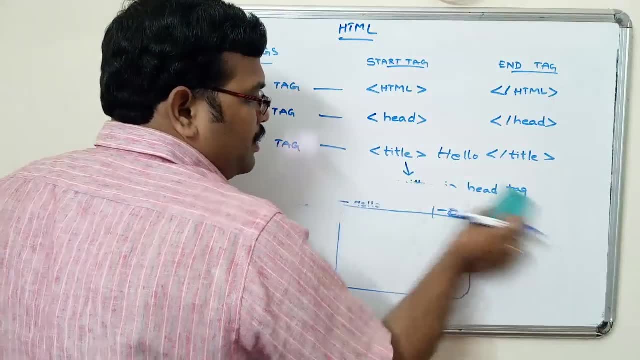 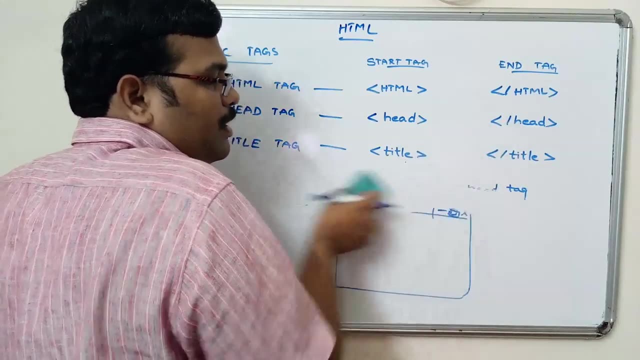 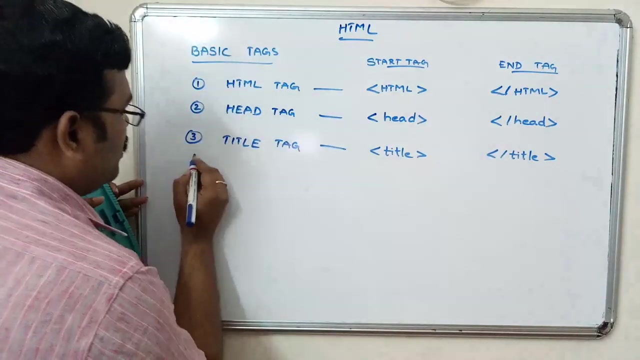 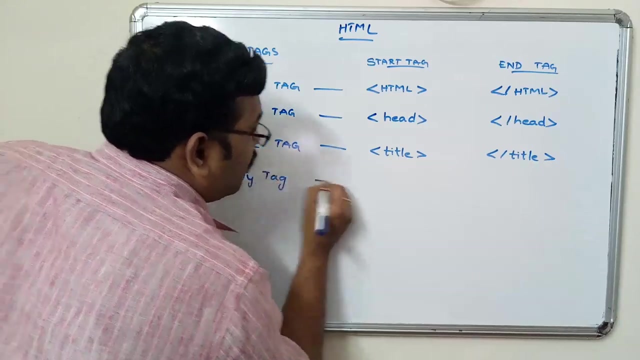 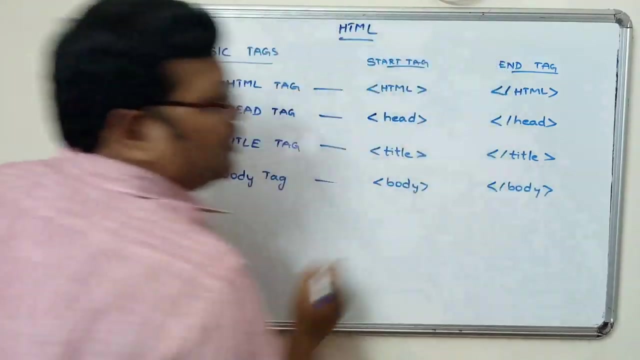 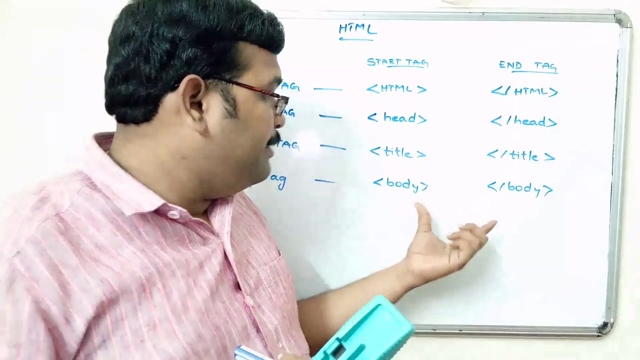 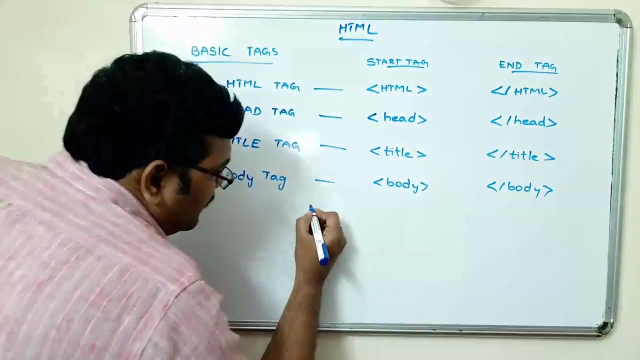 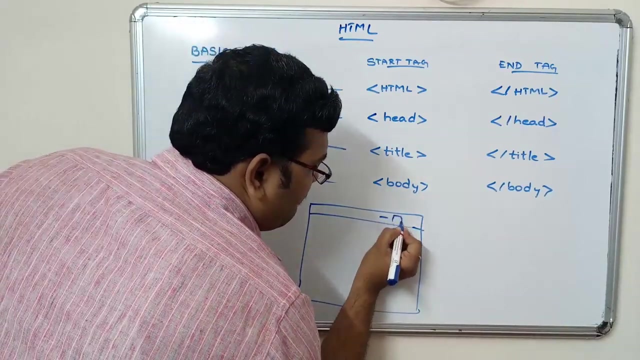 title bar. the title will be placed and this title should be written in between the head tag. what it is, see body tag is the actual content to be displayed. that means, whatever the text we are writing in between this body tag, that will be displayed on the web browser. so we know that. so if it is in a browser, so this is the title. 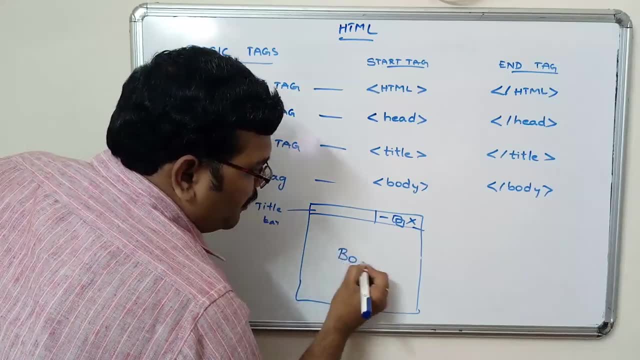 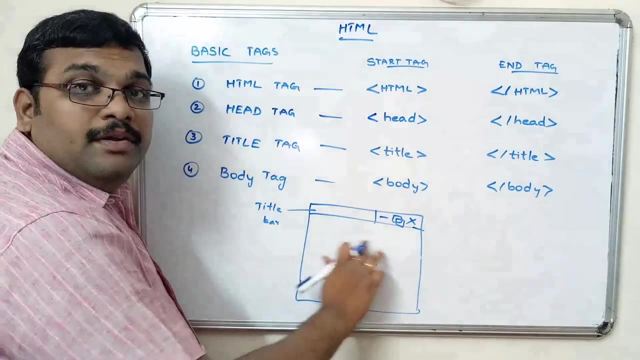 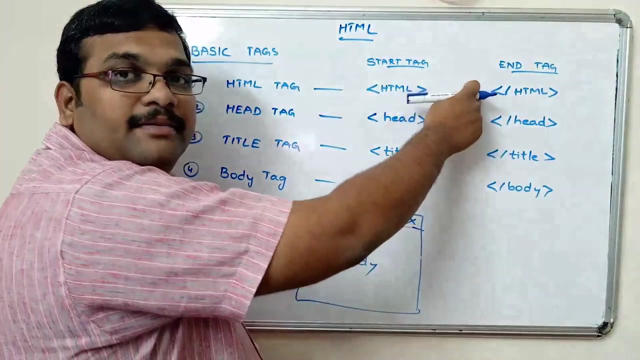 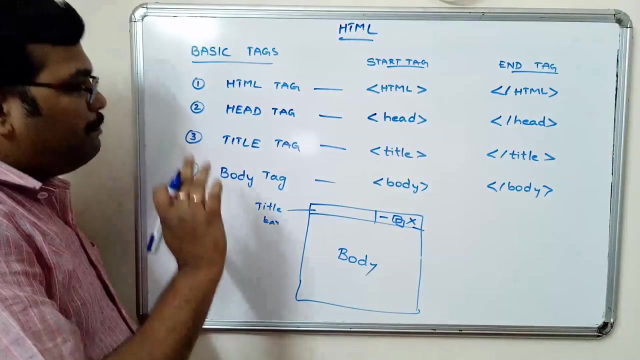 bar and this is the body. so, whatever the text we are writing in between this body, that will be displayed in this portion, right? so all these three tags should be written in between the HTML tag, because this implies the document contains the HTML, right? so these are the four basic tags we are supposed to write in every 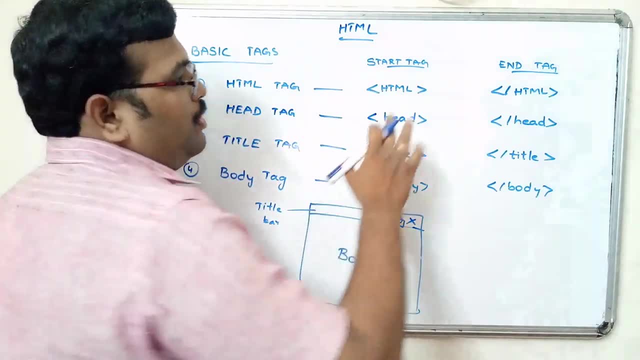 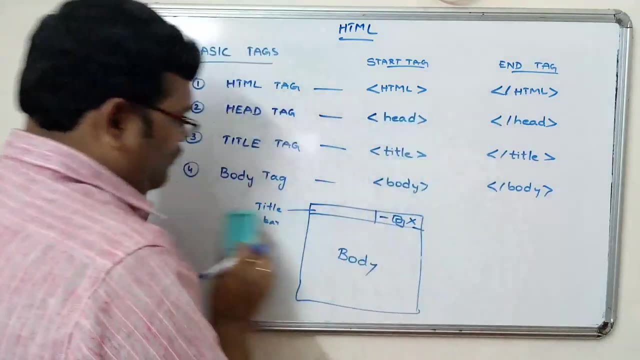 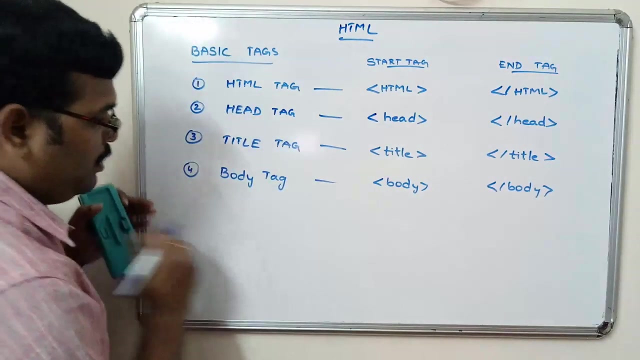 web page creation, right. so first of all, HTML tag, head title and the body: see. let us see an example. so paperwork: instead of picking the body tag, it is it communication tied to, and text editor next. so, if you like it, so when you would, often we would want you to. 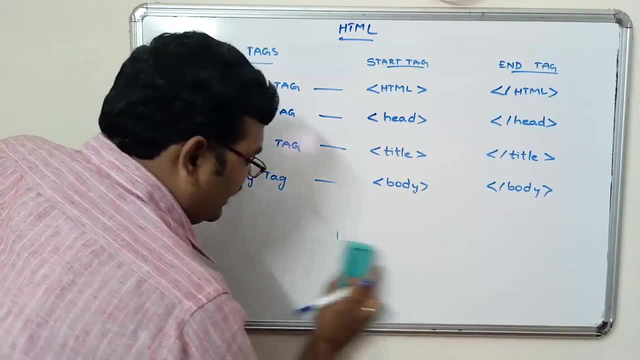 perfect me, because if it has a different text title, then it is actually the other way around. it would be better if you don't like it. but first of all, this is thepre jazzw тобou screen. in today's video, I have again practiced for you more about a way to 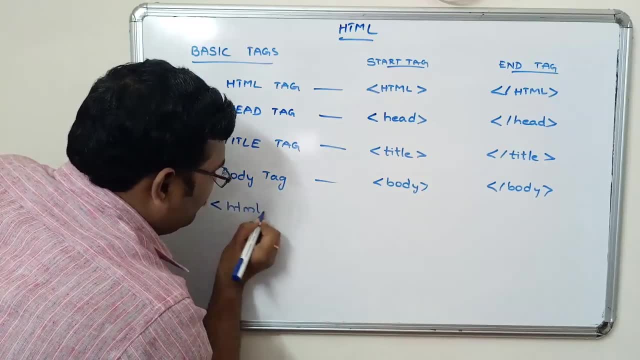 turn text into text. so I am trying to really showcase this again. so I've got all the way up. I've got the whole things in it- different types of buttons- so we will also have some Cayman as well, which are the ones that we are going to. 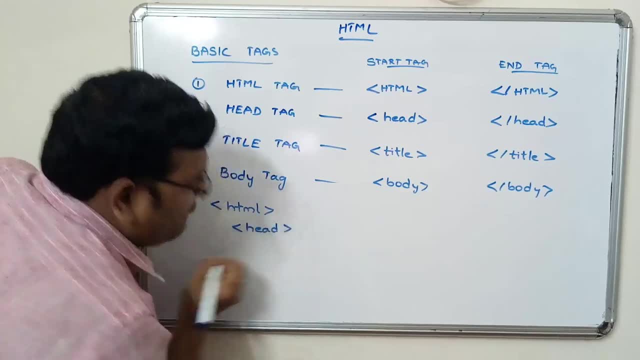 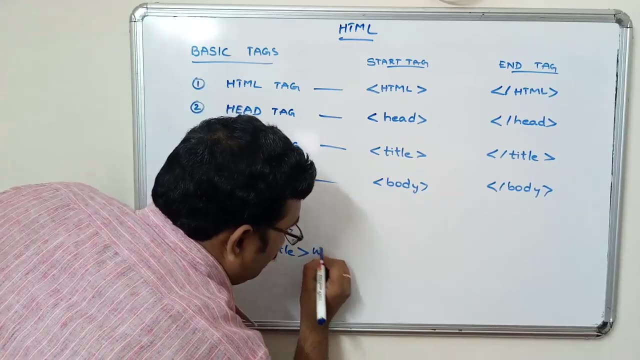 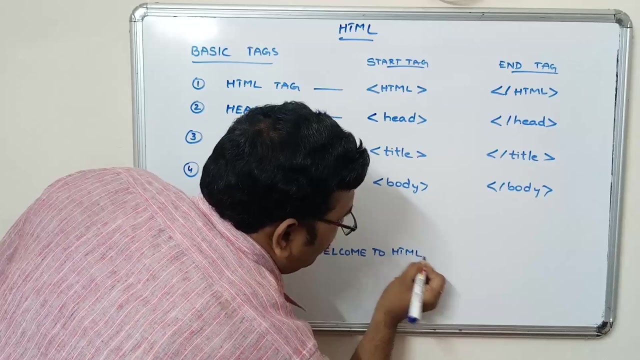 come back to in second place. so what I will be doing, the first thing is we will be comparing freue-file and we are going to see, for example. so I have прور and of course we have done all of the methods we have: writing title- welcome to HTML and closing the title right, starting that. 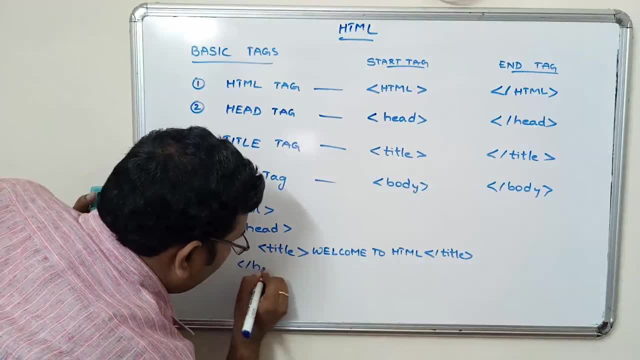 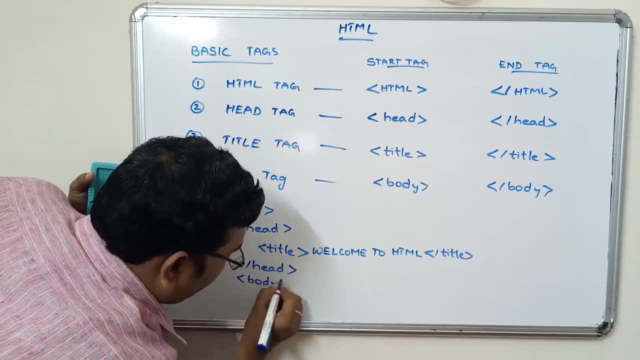 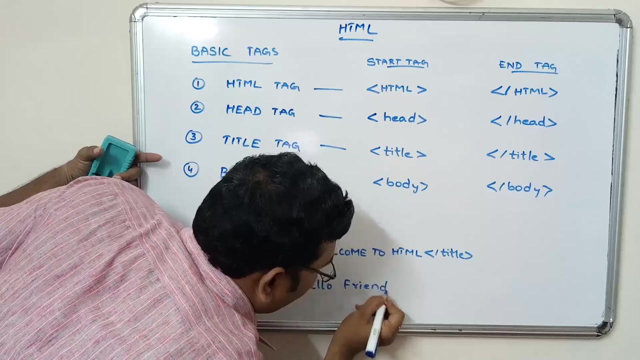 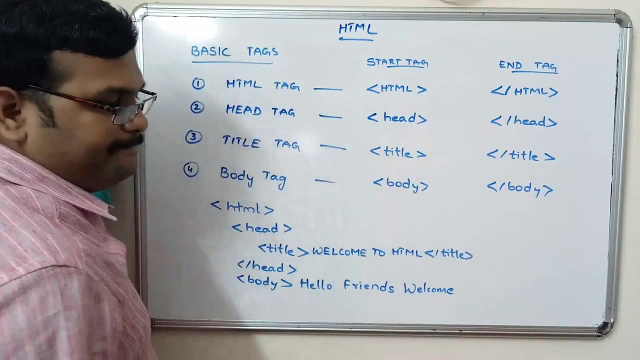 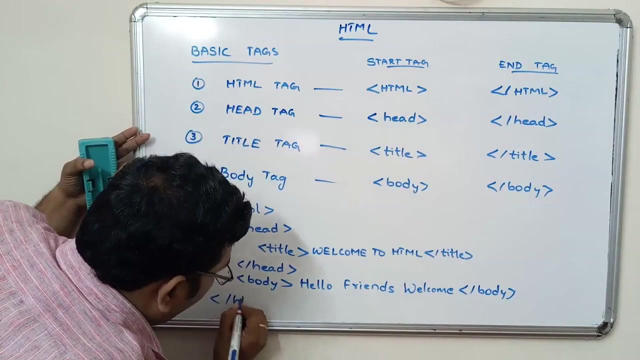 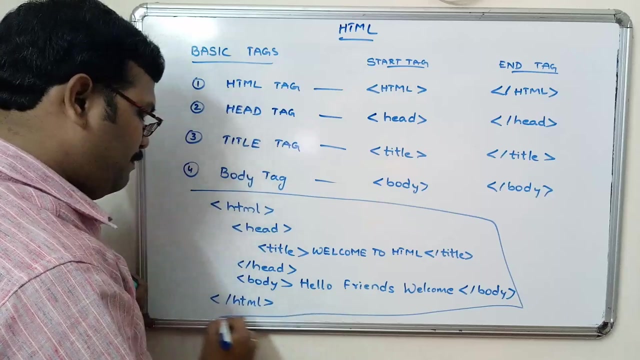 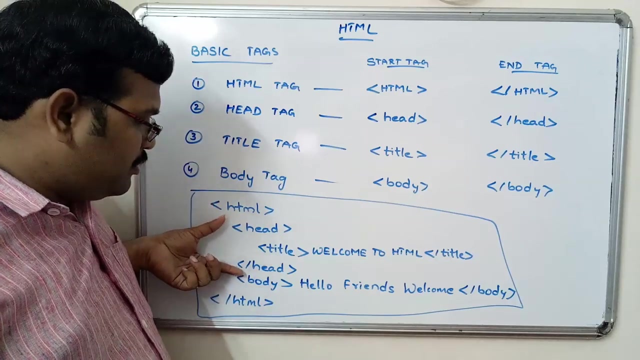 any day. and closing the head. now I am starting the body. hello friends, welcome. close the body and close the HTML. so this is a simple example, right so? this is a simple example, the first program, right? so HTML. in between the HTML, we're writing everything. so in between the head, we are writing the title. so in between the body. 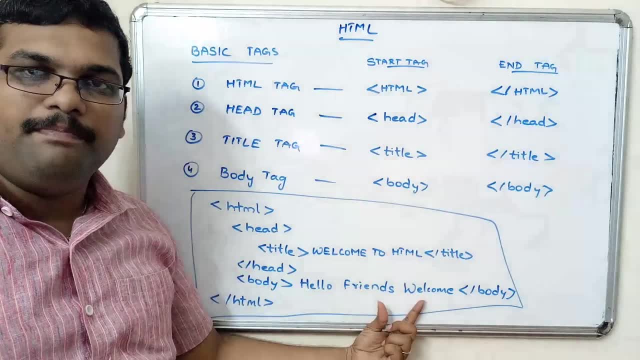 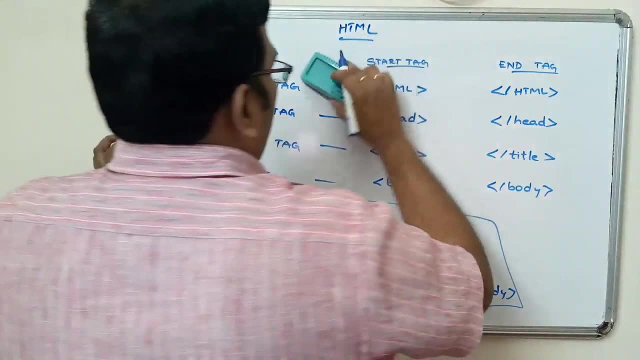 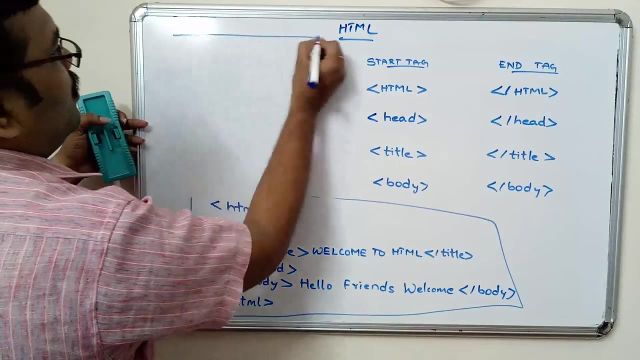 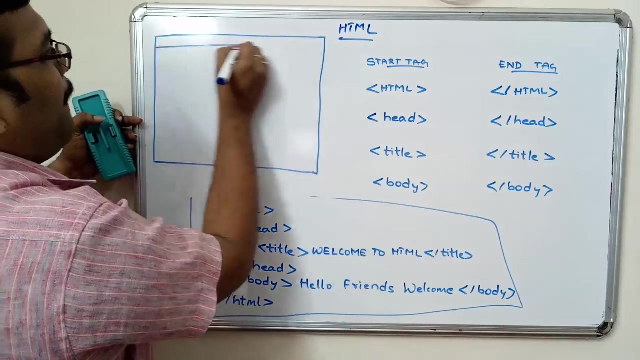 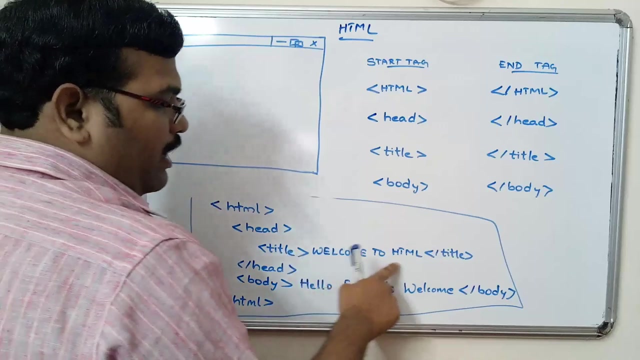 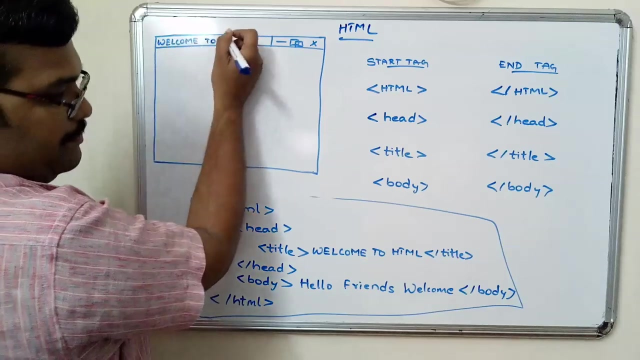 we are writing the text to be displayed on the web browser web page. see what is the output of this one. let us see here. let it be. this is a web page, so here we're writing the title: welcome to this channel. that will be displayed here. welcome to.